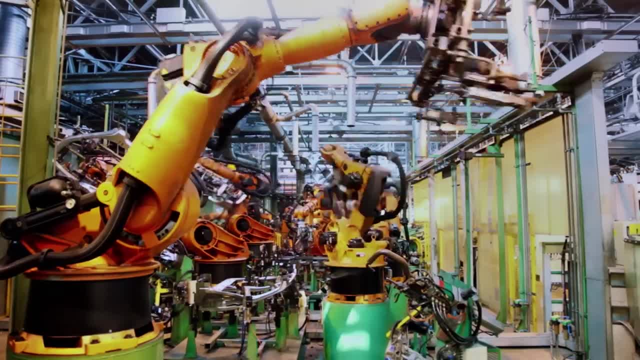 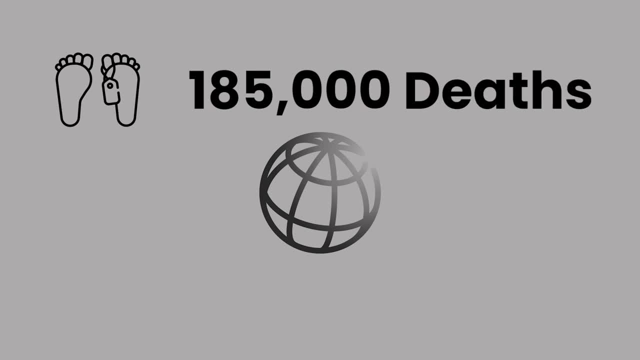 and the fastest growing end use of energy in most developing countries. According to the World Bank data, almost 185,000 deaths can be directly attributed to vehicular pollution. annually, Another 1.25 million people are killed and up to 50 million 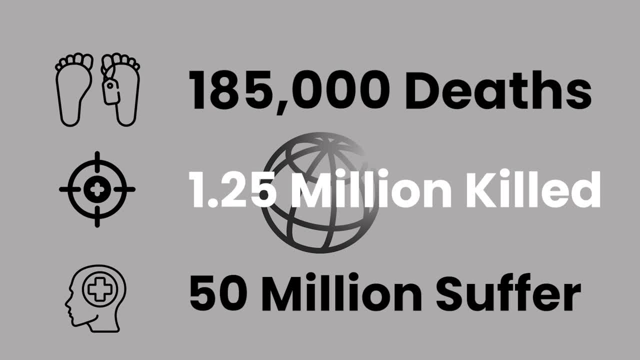 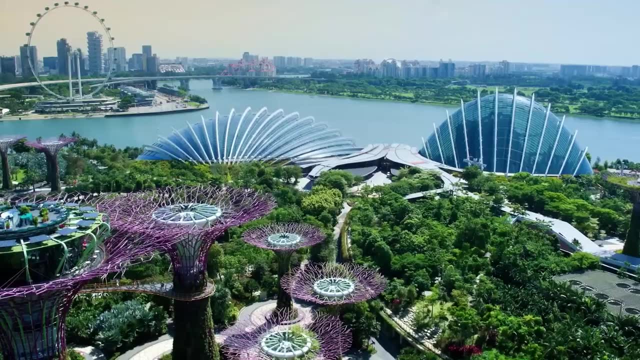 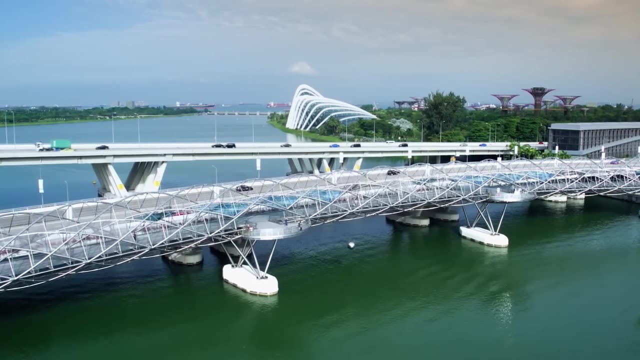 people also suffer injuries on the world's roads every year. The world's transport system has now undergone over two decades of technological advancements that have made transport services today much faster, eco-friendly and more accessible than they used to be. While all modes of transport undeniably need energy, it's become of utmost importance to 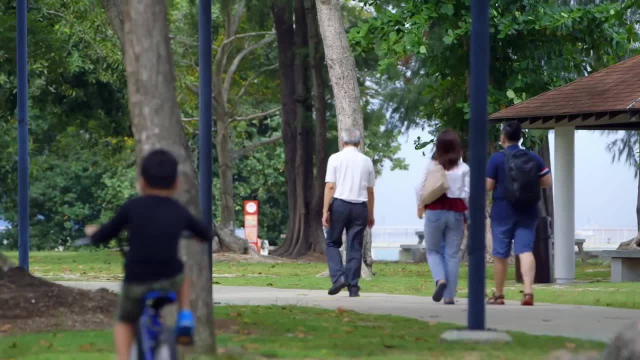 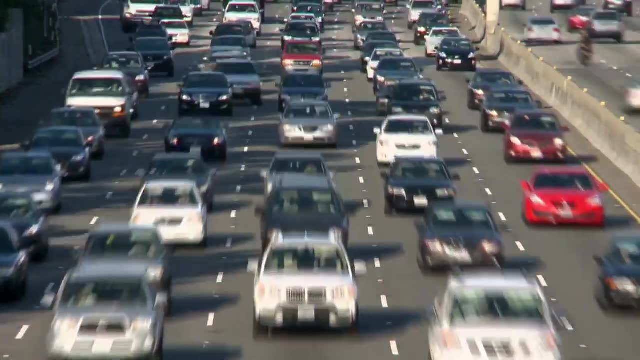 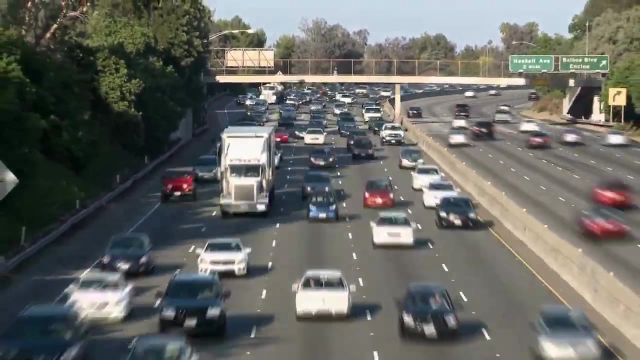 prioritize the use of environmentally friendly transport infrastructure that greatly reduces human carbon footprint. In many developed countries, people are increasingly gaining access to multiple transport options. In the developing world, likewise, the demand for mobility for people and goods has continued to grow significantly over the years. 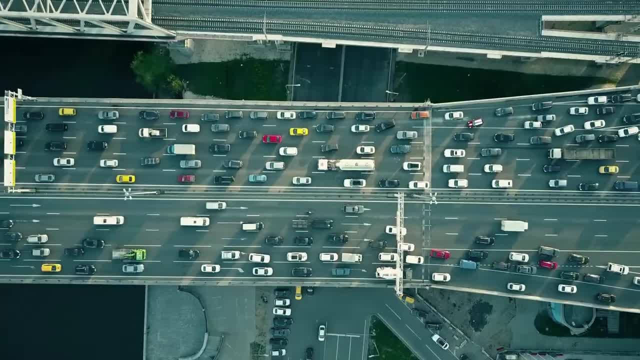 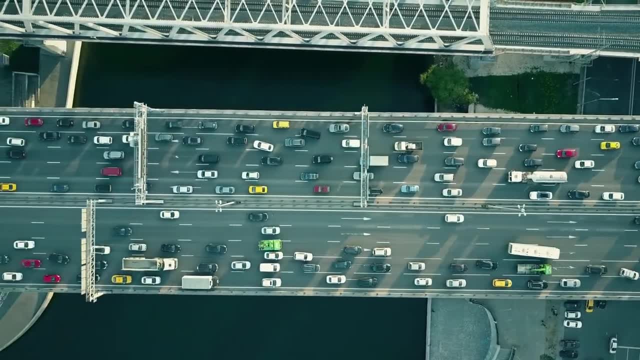 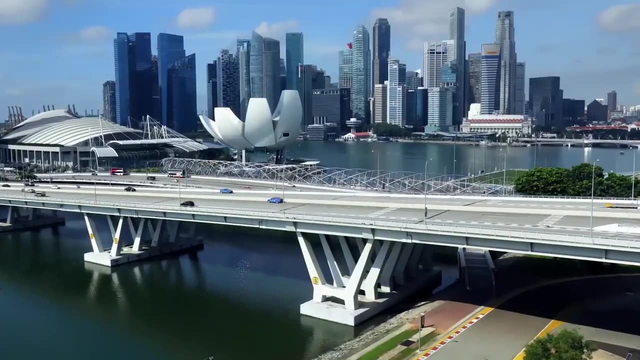 In both cases, developing and efficient, sustainable and eco-friendly transport networks that will serve a vast population of people and improve urban mobility has been a top priority globally since the turn of the 21st century, With sustainable and eco-friendly transport systems and technologies being highly self-reliant. 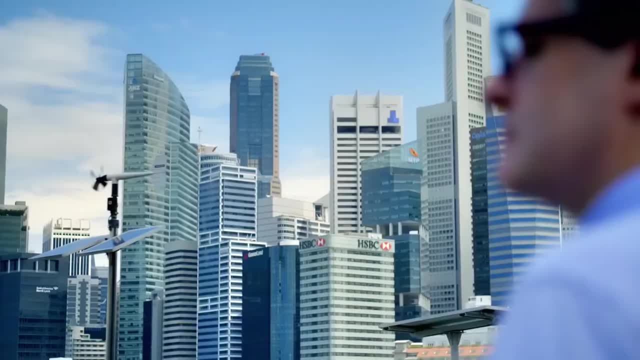 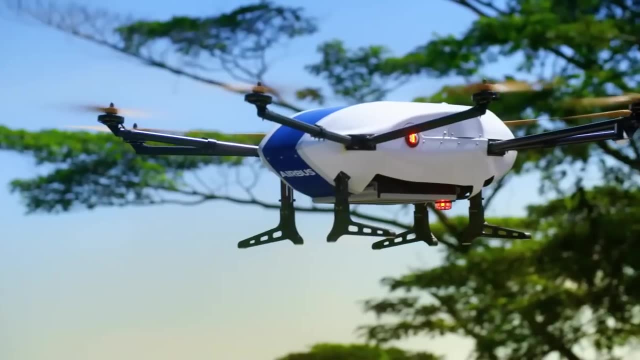 and having little to no negative impact on the environment. they have become the obvious route to addressing the many challenges of the old transportation systems. Here are some of the top innovations and technologies that are fast making transport better and more eco-friendly. Here are some of the top innovations and technologies that are fast making transport better and more eco-friendly. 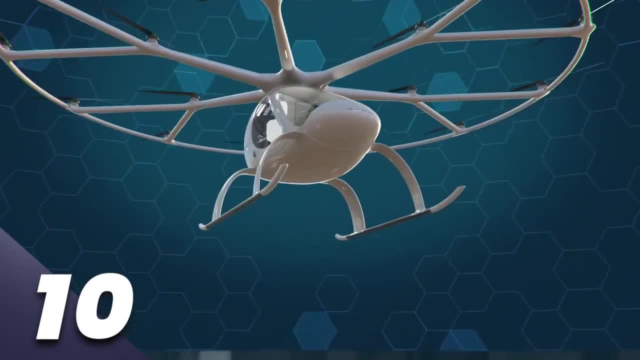 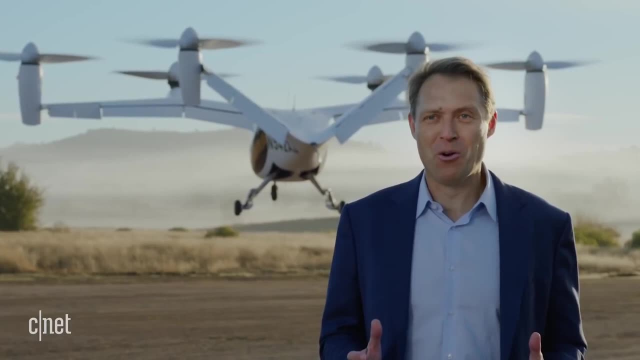 Here are some of the top innovations and technologies that are fast making transport better and more eco-friendly. Number 10. Helicopter Taxi. Helicopter taxis have fast become a popular mode of transport in developed countries. It is no longer an exclusive technology that is only used by rich and powerful people. 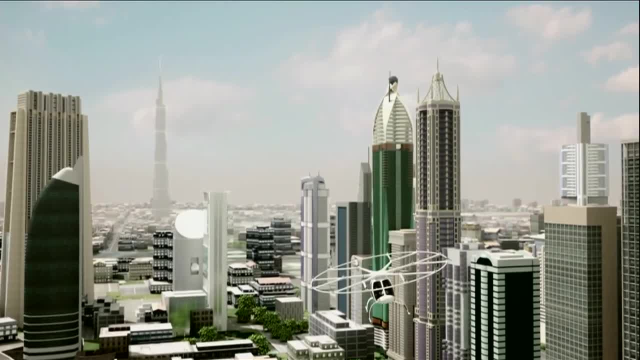 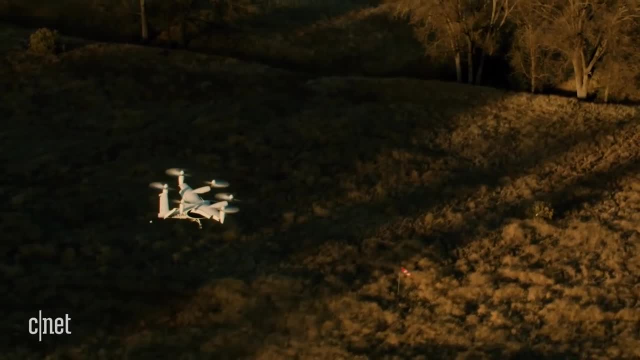 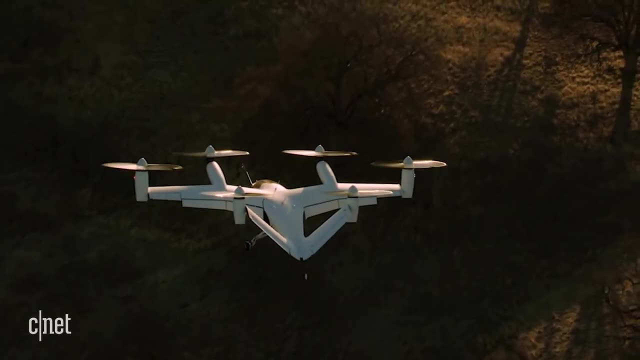 now vastly used in cities across America, China, Dubai and in many cities across Europe. This modern transportation offers a robust and versatile way of traveling for commuters. While a lot of helicopter taxis still run on none, renewable energy- innovations in renewable energy- are fast getting incorporated into 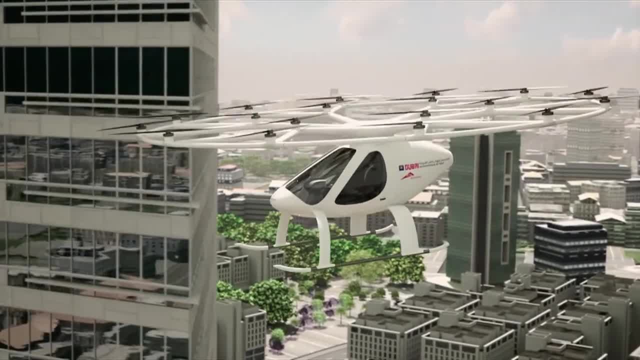 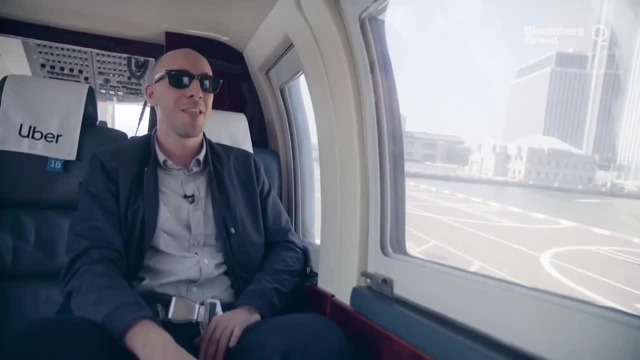 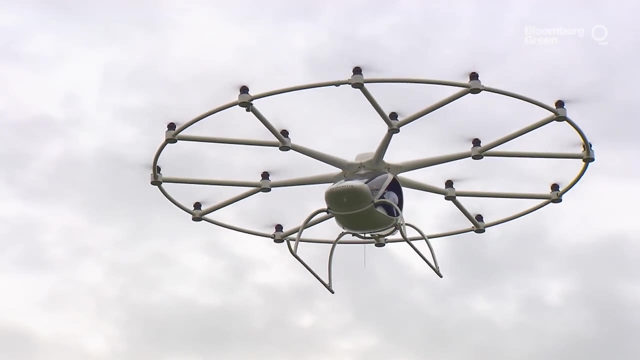 building technologies for helicopter taxis. Helicopter taxis provide you with spectacular sightseeing, making it the perfect technology for a sightseeing tour. The large windows allow you to enjoy the spectacular aerial view and get amazing photos for a quality travel experience. Ever dreamt of being able to visit multiple cities in a day? 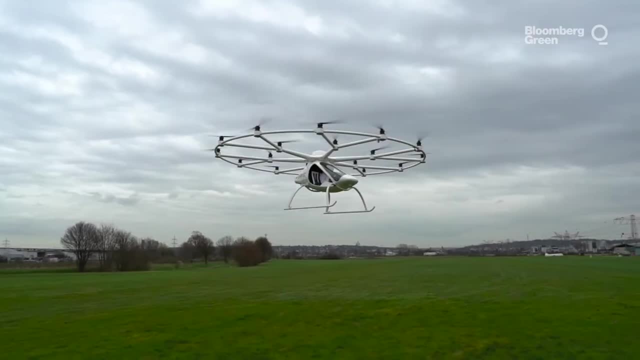 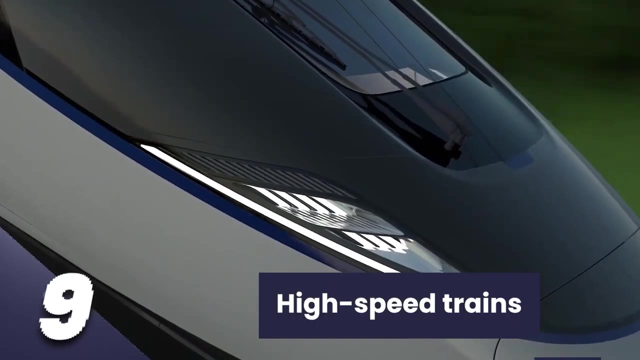 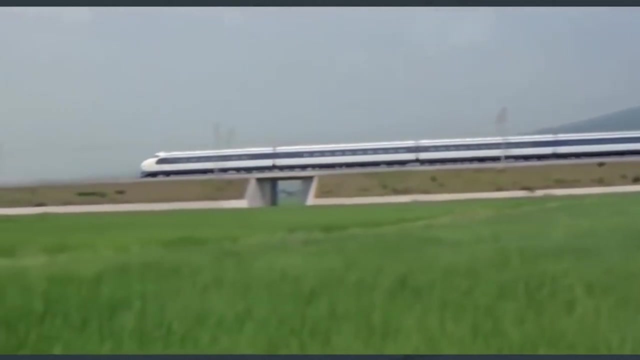 Helicopter taxis travel at top speed and make this possible with great comfort and convenience. Number 9. High-Speed Trains. High-speed trains are one of the most effective and sustainable modes of transportation because these trains function with renewable energy sources. This means zero emission into the 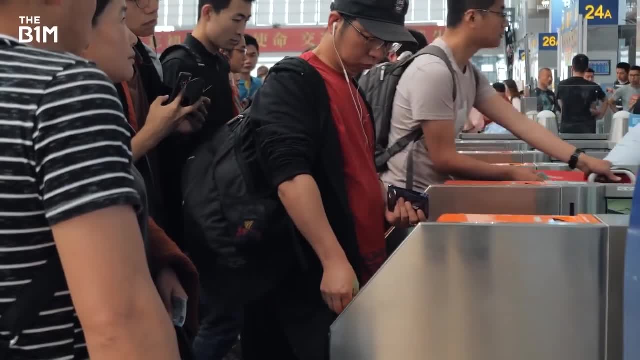 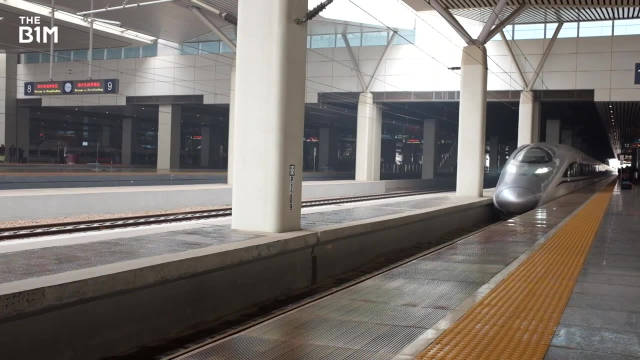 atmosphere, and they can accommodate more passengers than buses or cars. High-speed trains are also known for their speeds, as some reach up to speeds of 220 miles per hour. These trains greatly help in relieving some of the traffic jams in congested cities across Europe. 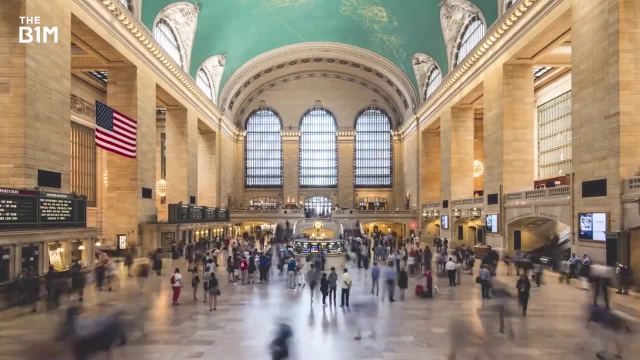 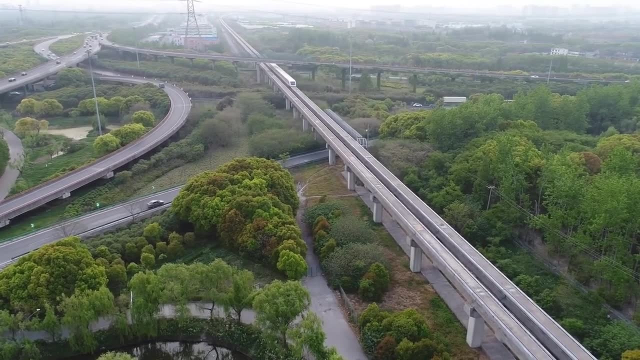 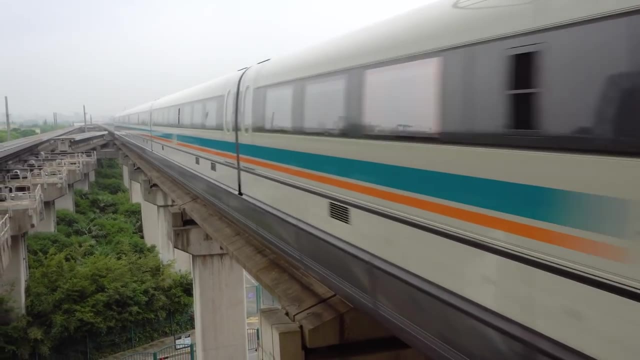 Asia and America, where they are widely in use. These trains are completely safe and are presently one of the safest forms of transportation in the world. If you are the busy type, riding a train will help free up time to focus on getting more work done. The high-speed train by far is the most common sustainable mode of transportation. 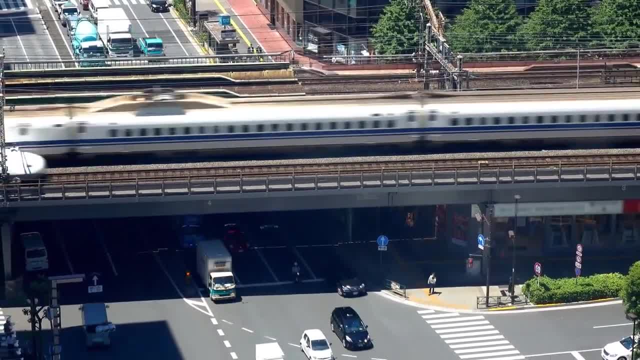 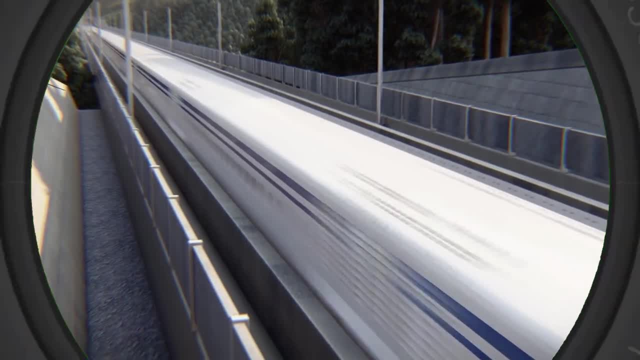 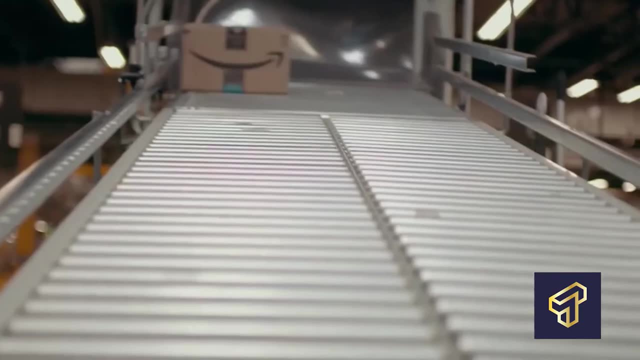 in urban cities. Cities like China, Japan and Korea have especially been able to successfully utilize and integrate the benefits of high-speed trains Number 10.. High-Speed Trains- Number 8.. Innovations in Parcel and Freight Delivery: Big multinational courier services as well as medium-scale courier enterprises. 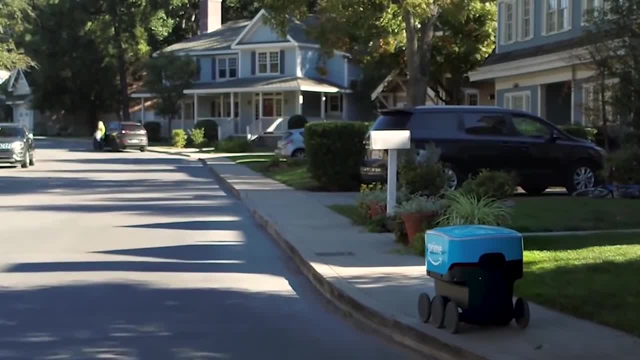 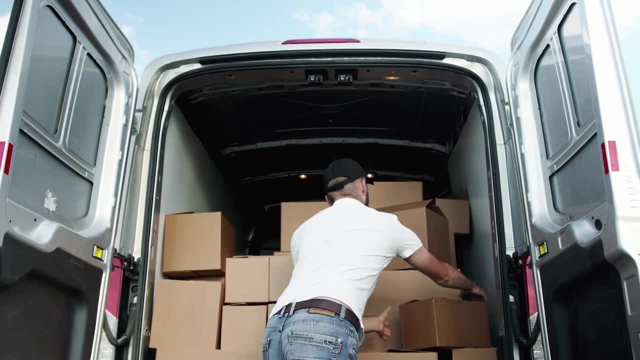 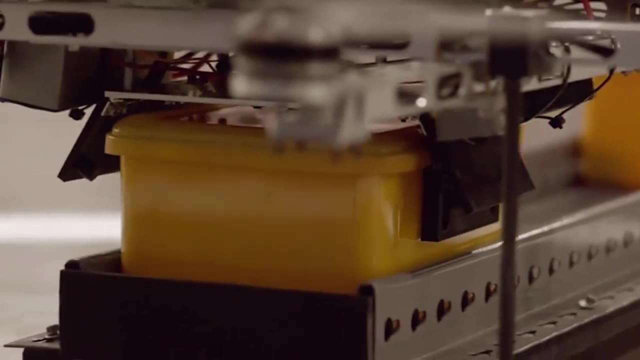 are now adopting the use of electric scooters and e-bikes for fast delivery transportation. There has been an increase in demand for food and parcel deliveries following the pandemic, and some courier services use their technologies to keep up with their demand. More importantly, these innovations are sustainable, eco-friendly and have zero carbon. 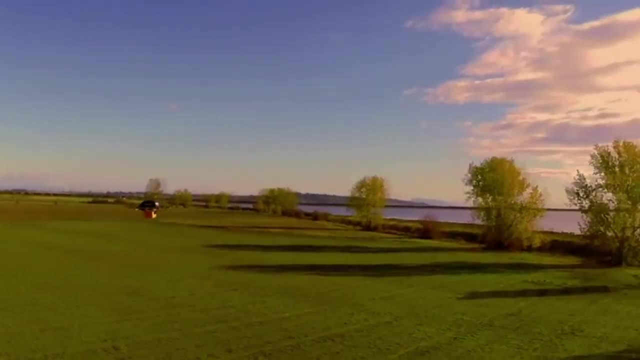 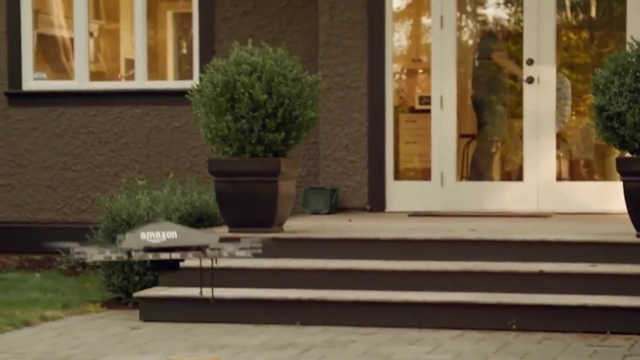 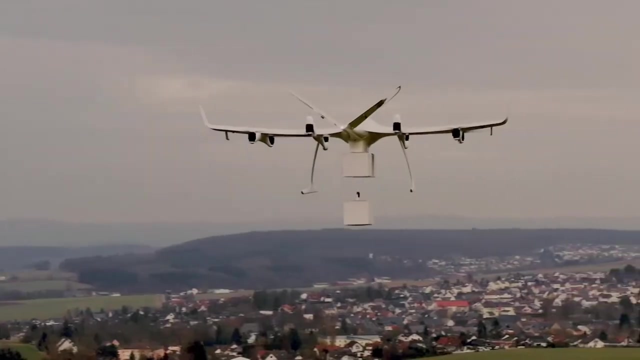 emissions. Another innovative technology in the courier industry that has revolutionized the mode of delivery is the adoption of drones for express delivery. Many courier services are already experimenting with the use of drones because it offers the potential to provide fast and easy deliveries to congested areas and to rural areas that might be difficult to access by train or 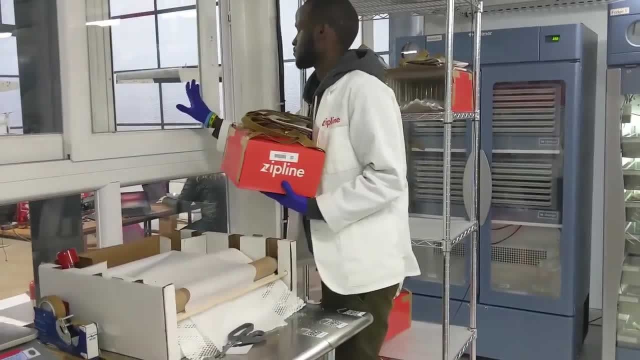 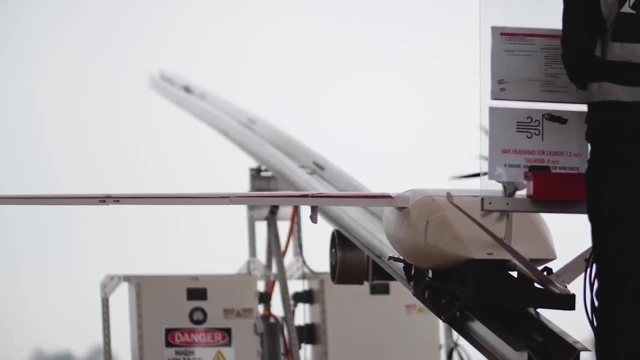 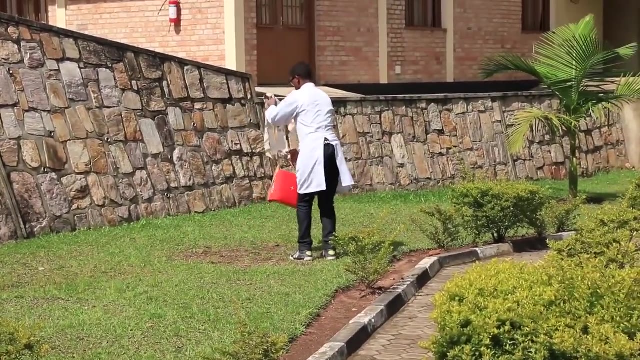 vehicle. For instance, UPS, a major courier service provider, has partnered with Zipline, a startup, and is focusing on medical drone delivery to deliver medical aid in Africa. Drone delivery is also widely considered as the future of e-commerce, given the potentials that it holds. 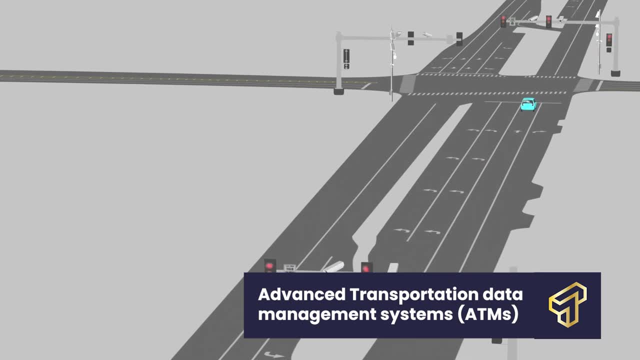 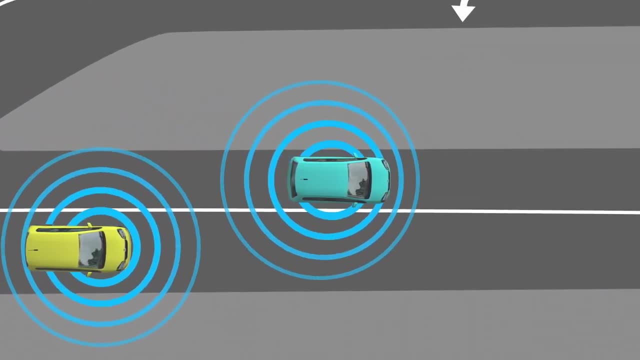 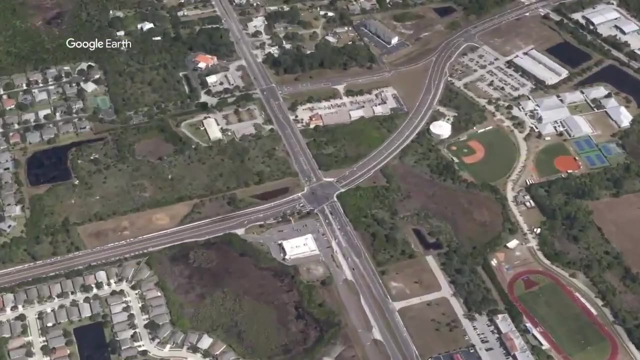 Number 7. Advanced Transportation Data Management Systems. Most developed countries make use of ADMs to manage highway traffic through real-time information collection, processing, analysis and dissemination to concerned stakeholders. You can think of it as sophisticated software program that enables authorities to monitor the transportation network and highways by various 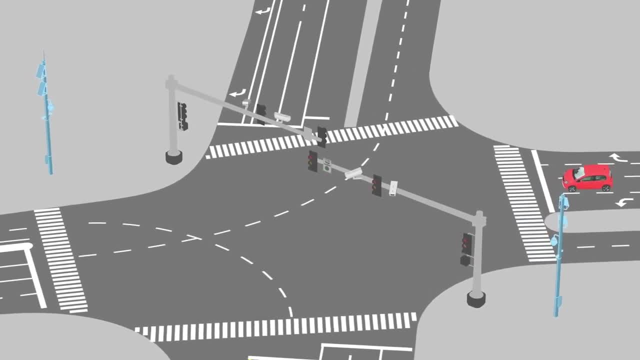 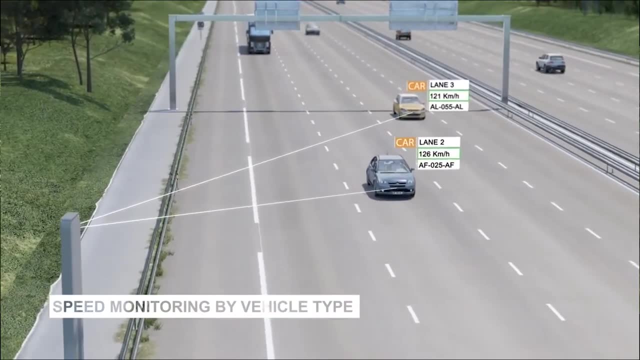 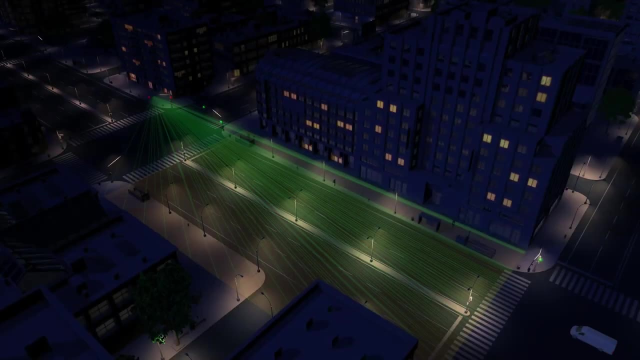 sensors and technologies to create corrective measures that will guarantee the assurance of safety for road users, enhanced efficiency, productivity, mobility and a better traffic management system. If you've ever sped past a red light, especially when nobody saw you, but you ended up getting a ticket and you wonder how you were caught, The answer is: 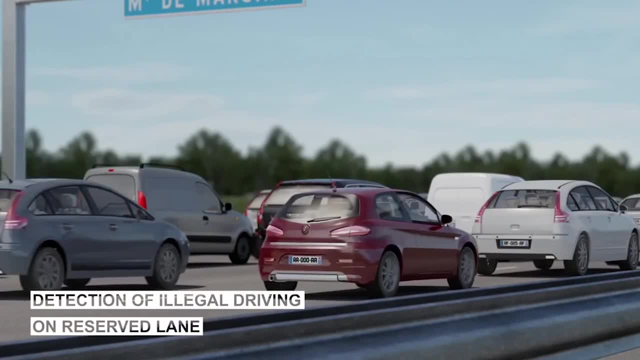 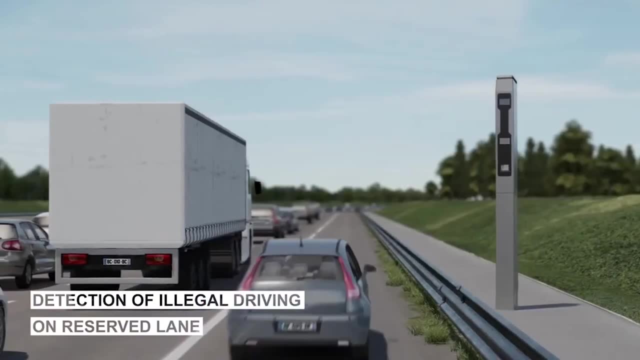 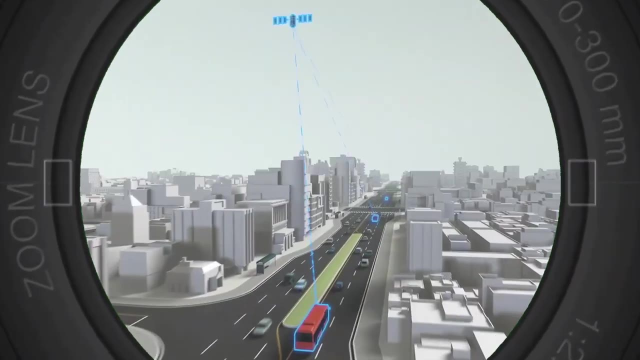 you were being monitored by the ADMs embedded in the traffic light. The ADMs work like an API that integrates different roadside equipment to generate its data. This might include data from surveillance cameras and other installed equipment by the roadside Number 6. Smart Transportation. 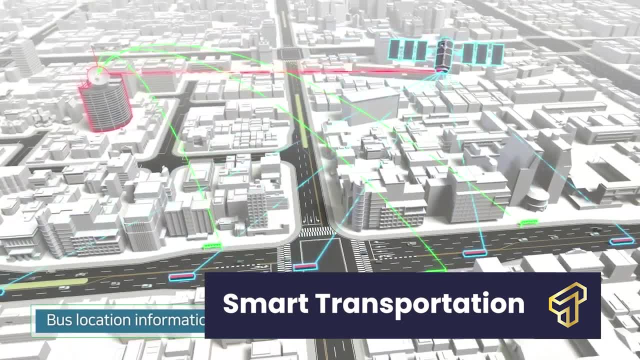 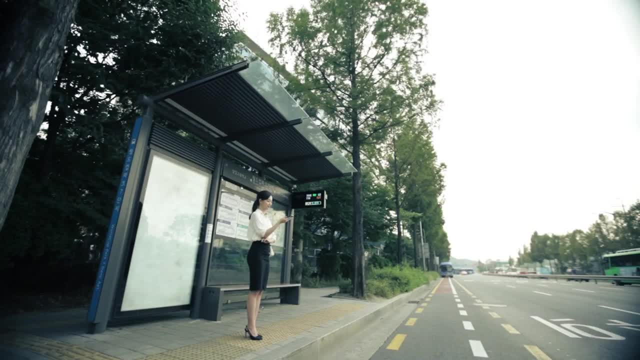 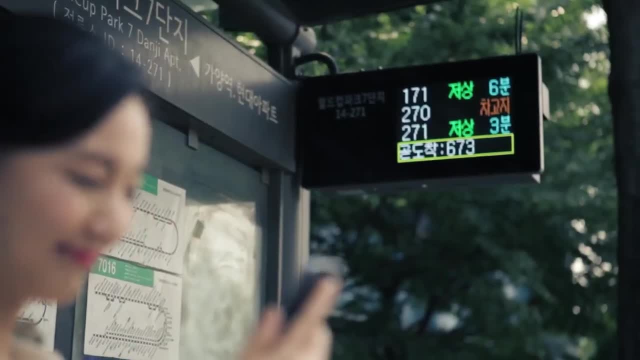 Most of the ADMs are based on the ADMs. Most of the ADMs are based on the ADMs, Most notably the use of car navigation. If you have ever boarded an Uber or Lyft, you would have made use of the inbuilt navigation system or app. 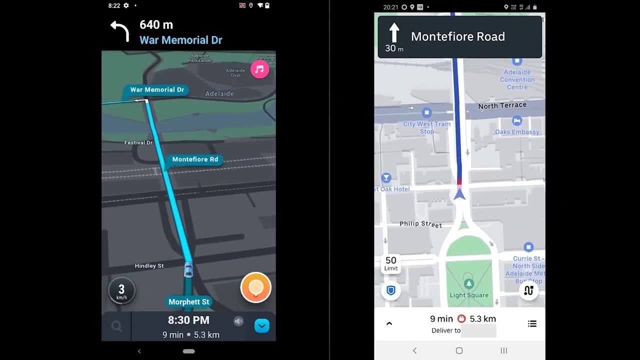 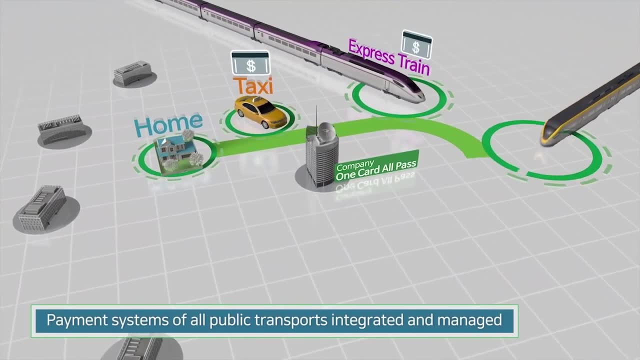 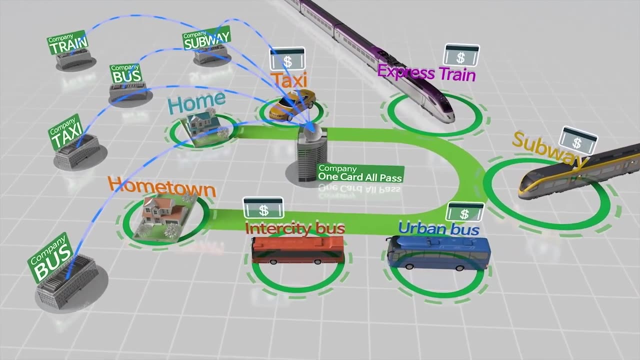 Well, this is also a part of smart transportation technologies that enables users to get position data, which is then correlated to the position of a vehicle on the road. This technology also helps to calculate routes when directions are needed. Another example of smart transportation technology is traffic signal control systems. These systems help. 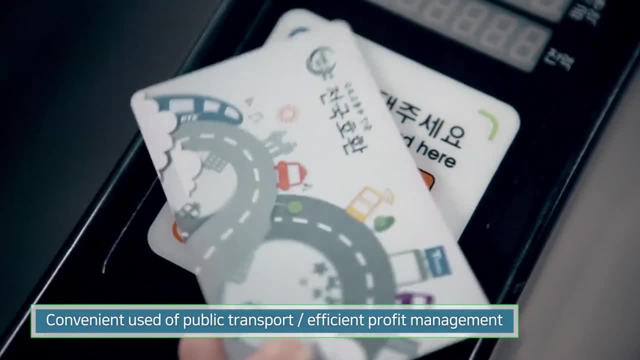 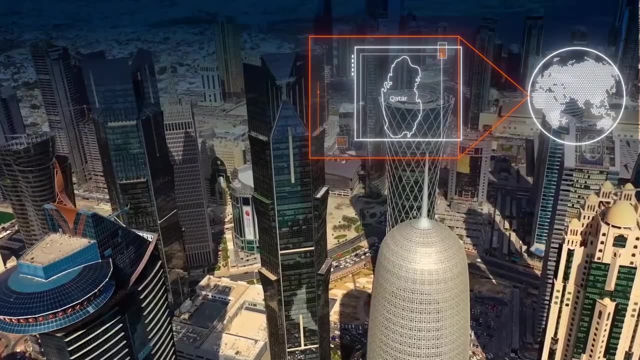 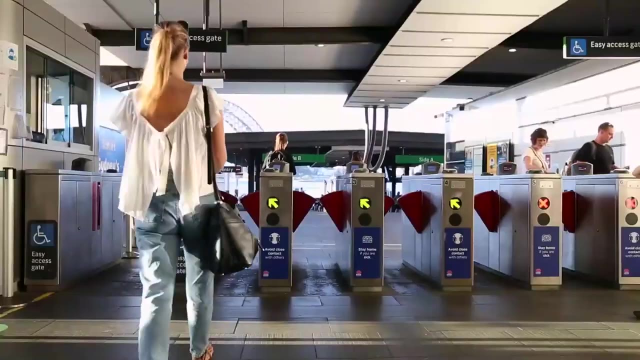 you, as a commuter and or a road user, to respond appropriately to your surroundings and adjust to traffic conditions. Another one would be speed cameras that use detectors to detect vehicles going above the legal speed limit. These are all smart transportation technologies being created to improve the process of transportation. 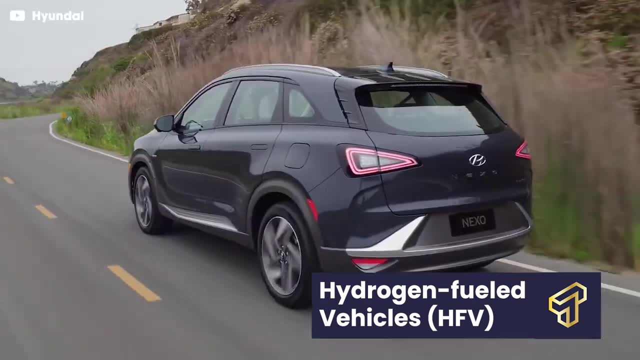 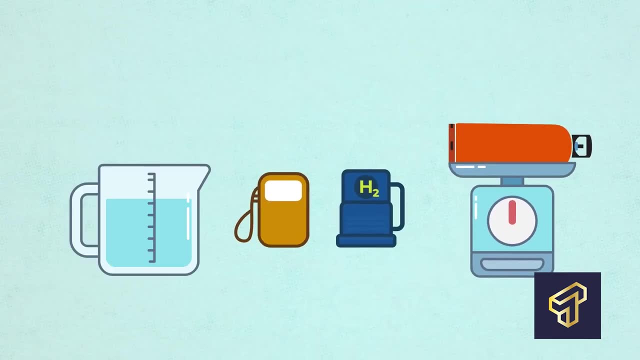 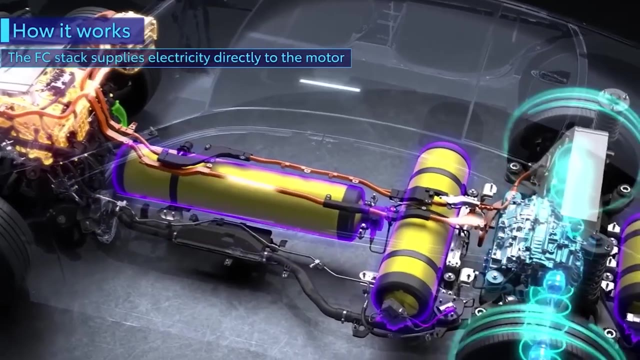 5. Hydrogen-Fueled Vehicles. You are probably thinking about a car that runs on water, especially with the word hydrogen in the mix. Well, a hydrogen-powered vehicle isn't technically a vehicle that works on water. HFV or fuel cell electric vehicles use a propulsion system like that of electric vehicles. 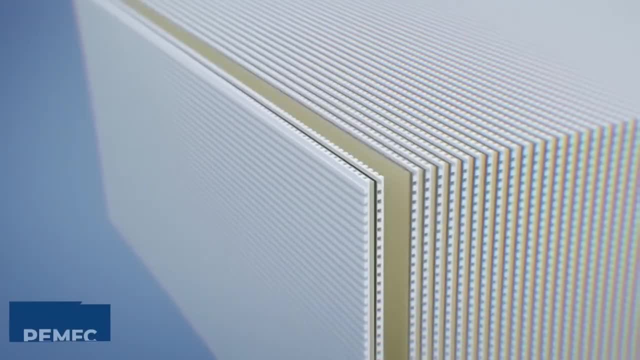 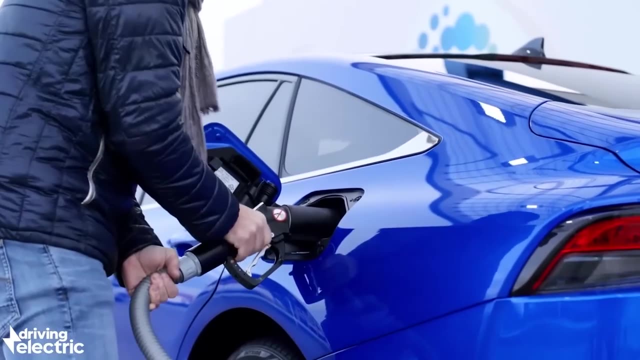 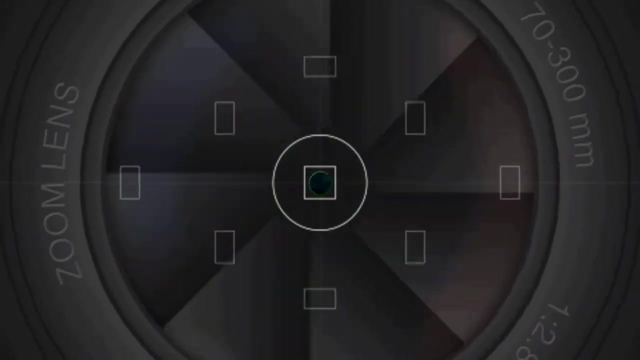 Because, unlike electric vehicles, the energy that is stored as hydrogen is converted into electricity by the fuel cell, And the good thing about these vehicles is that they produce no harmful emissions and are highly efficient when compared to other energy sources. 4. Electric Vehicles- 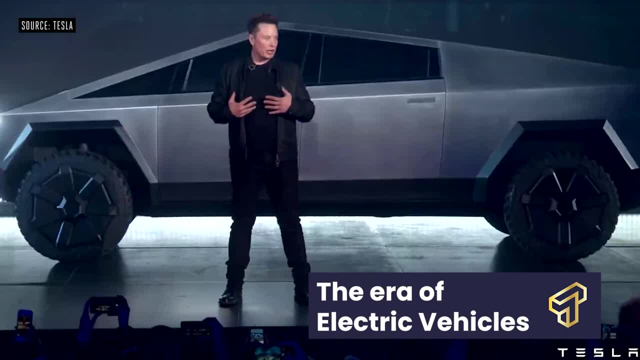 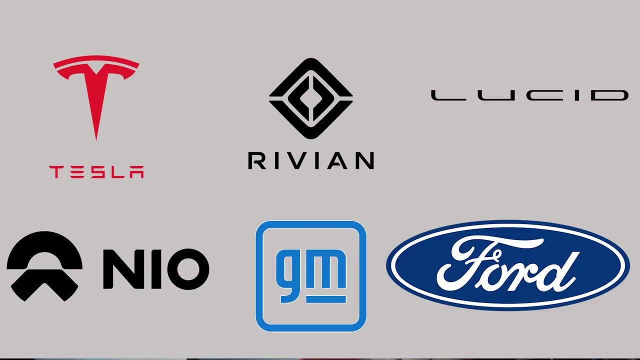 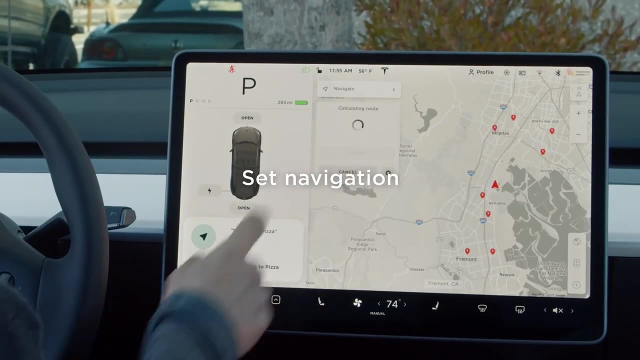 4. The Era of Electric Vehicles. If you ask me, I will say we are currently living in the era of electric vehicles because we have major EV brands like Tesla, Rivian, Lucid, NIO, GM and Ford, whose products have revolutionized the transportation industry. Electric 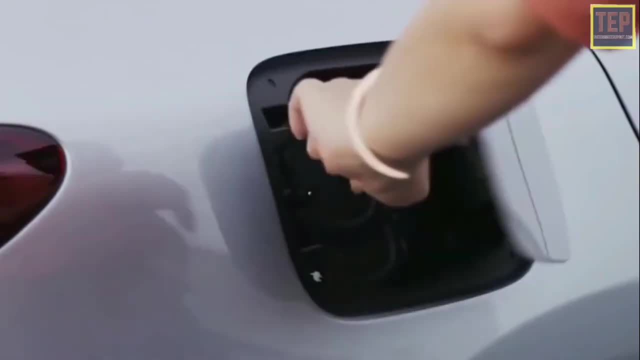 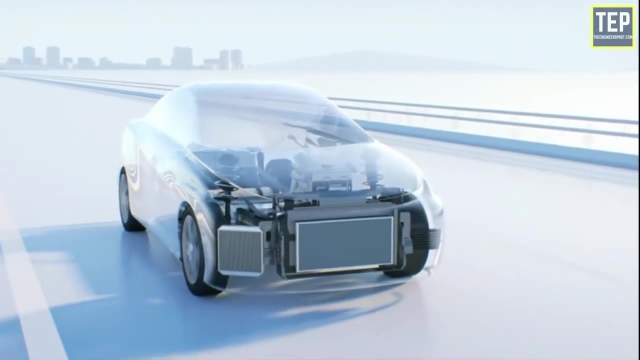 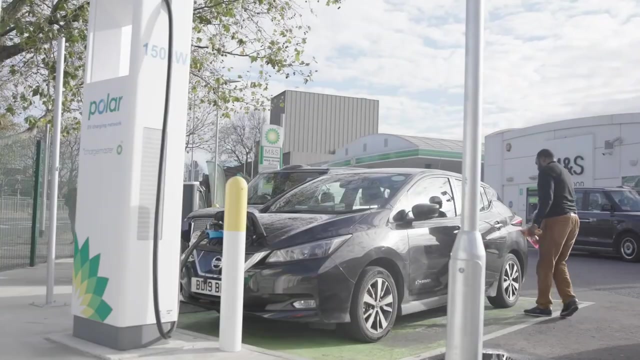 vehicles are vehicles that are fully powered on electricity. These vehicles have been proven to have low running costs, as they also are environmentally friendly and use no electricity. Some EVs, however, use lithium-ion batteries, as they have greater longevity and are excellent at retaining a large amount of energy. Another benefit of the EV is the fact that they are much. 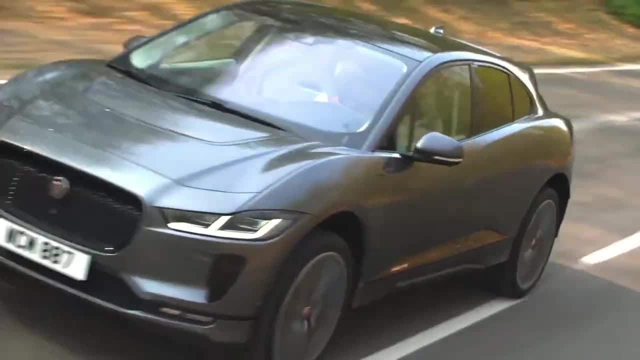 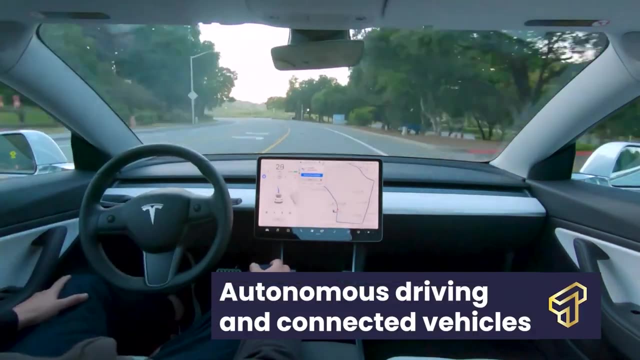 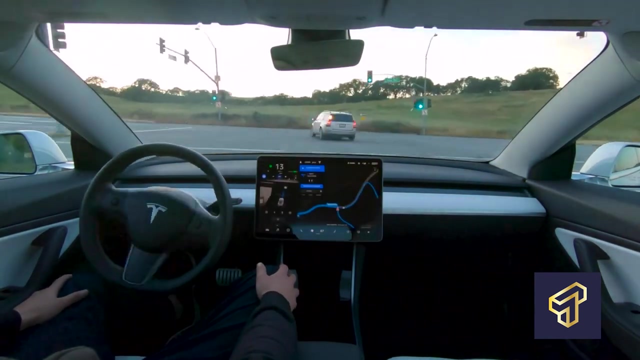 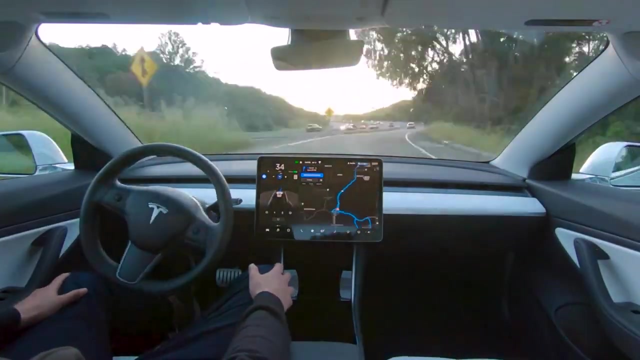 quieter than vehicles that run on fossil fuels, so you have less noise pollution. 3. Autonomous Driving and Connected Vehicles. Connected and autonomous vehicles, otherwise known as CIVs, are vehicles that combine connectivity and automated technologies to assist or replace humans in the task of driving. This is usually accomplished through a combination. 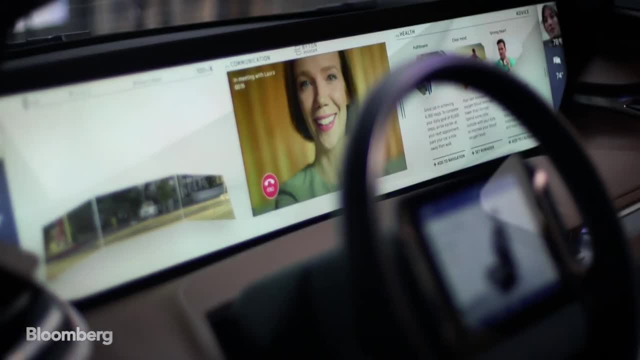 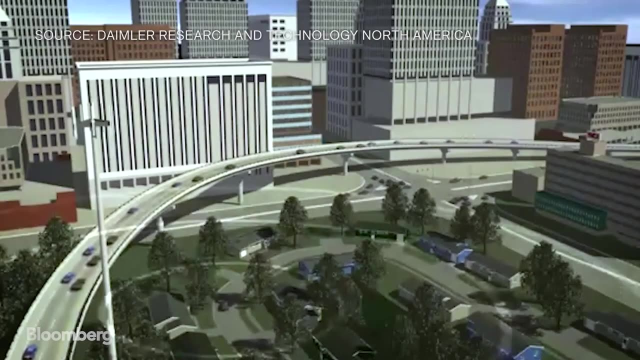 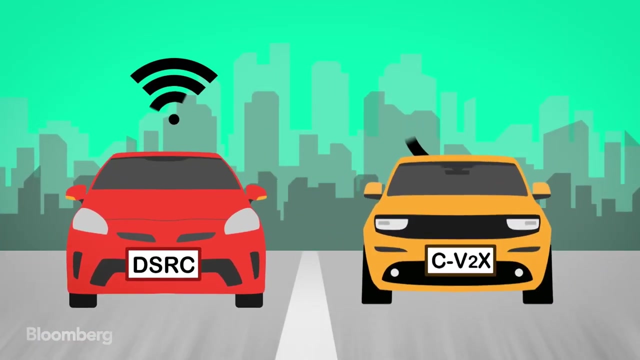 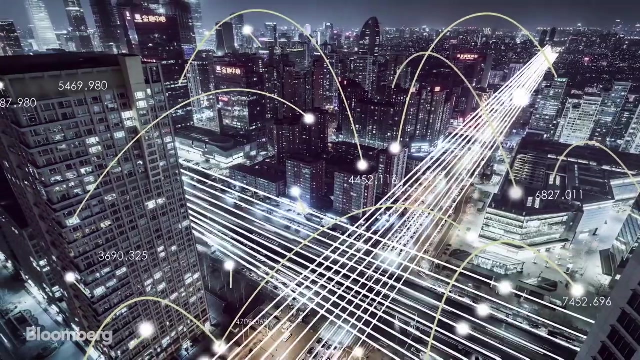 of advanced sensor and AI technology, onboard and remote processing capabilities and advanced telecommunication systems. CIVs possess the ability to save lives, because most road accidents are caused by human error. Another great advantage of the CIV is that it can interact and connect with other vehicles and share information with other sources to create 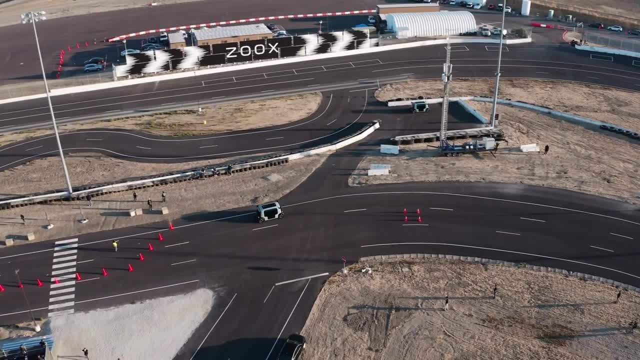 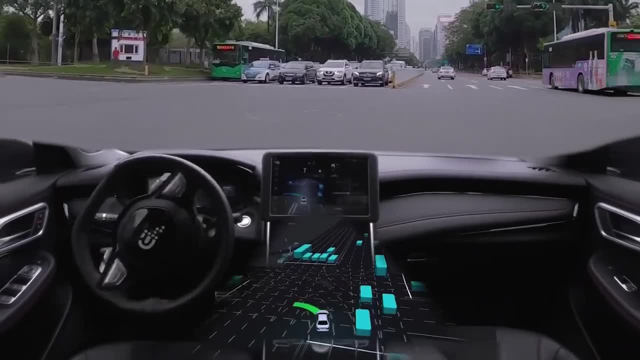 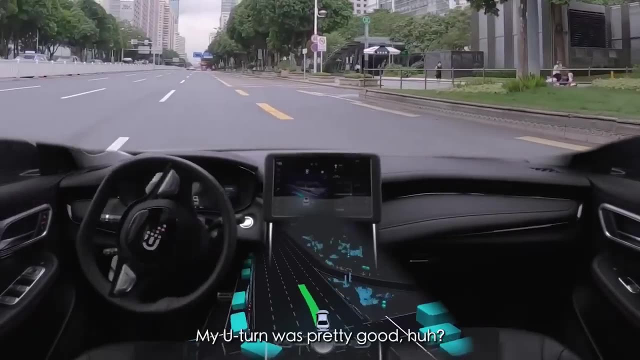 a better driving experience. What this means is that, with technology, CIVs can interact with multiple vehicles and systems such that they can play a significant role in road safety as well as traffic management. Fewer accidents will translate to less traffic congestion, which will in turn reduce emissions. 2. AI Assistance. 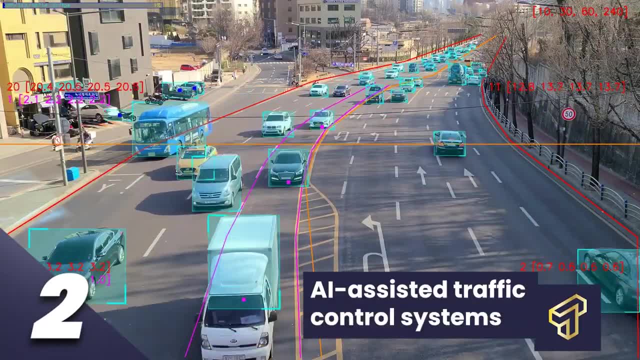 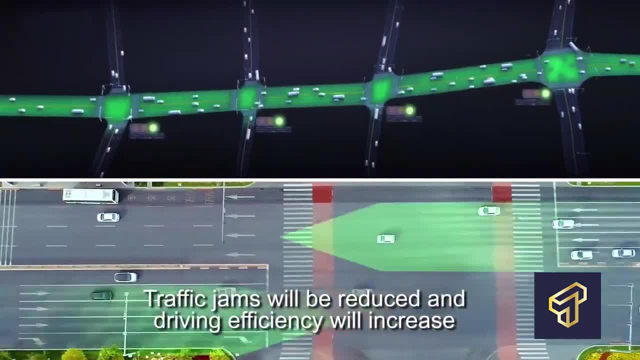 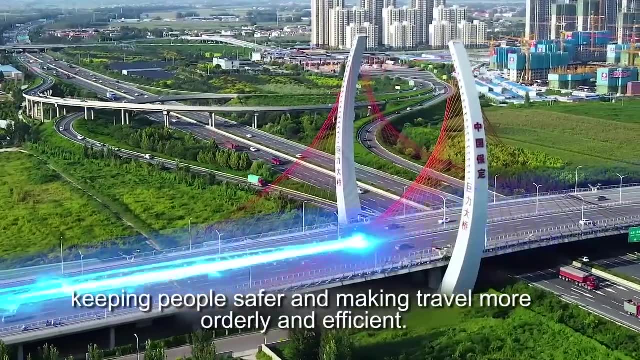 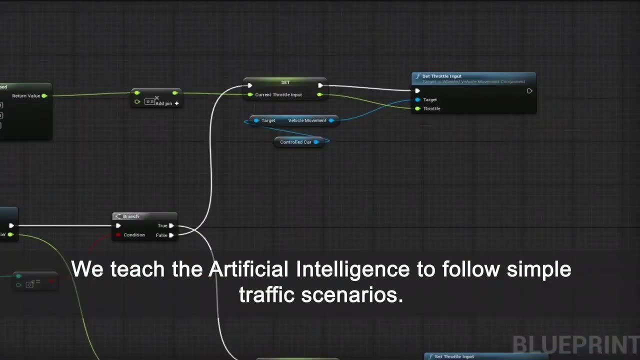 road traffic by reducing human error and speeding up the process of detecting and responding to an accident, thus improving safety. The ATCS also assists in determining and increasing efficiency during peak hours by optimizing the flow of traffic. ATCs work better in collaborative systems with ADMs. 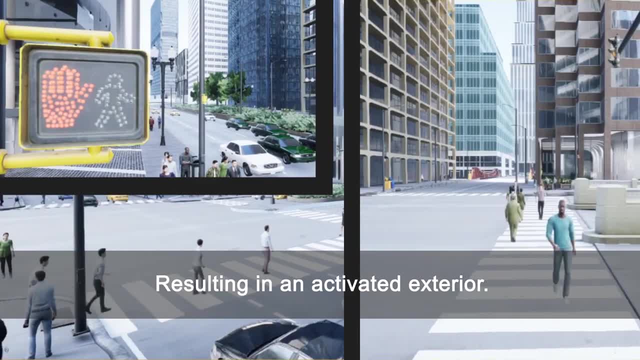 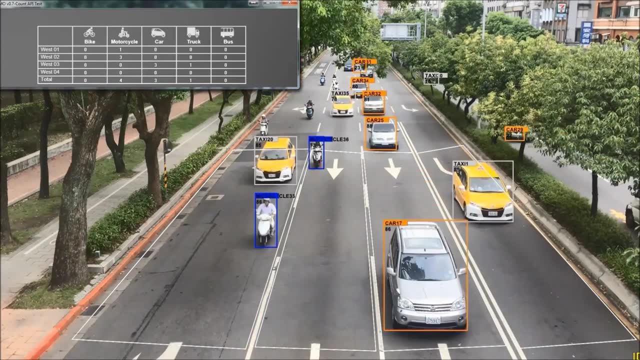 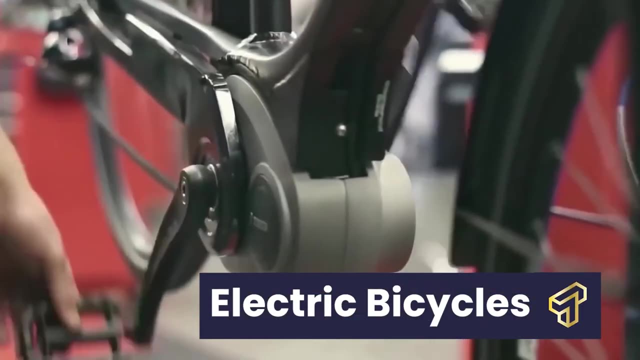 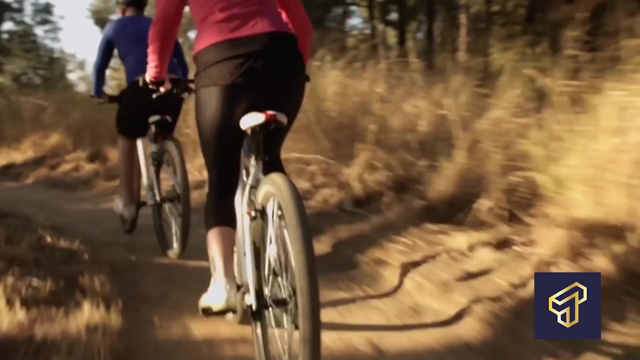 These traffic control systems also work like an API that integrates different roadside equipment to generate its data. This might include data from surveillance cameras and other installed equipment by the roadside. 1. Electric Bicycles: Electric bicycles or e-bikes are motorized bicycles that come with an integrated electric motor used to enhance propulsion. 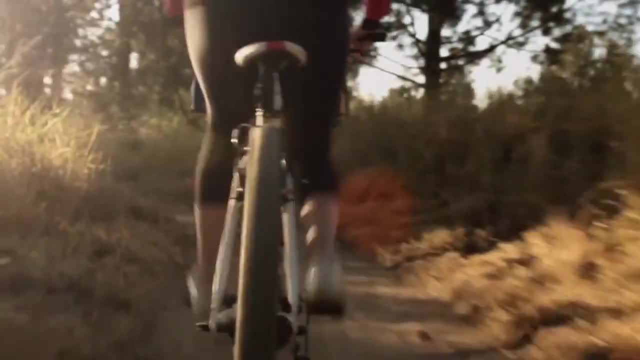 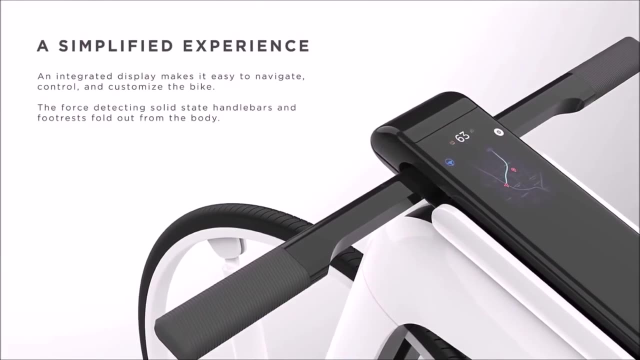 The difference between a conventional bicycle and an electric one is that you can cover more distance with it- E-bikes- without getting fatigued or stressed. With e-bikes, you also don't have to worry about difficult terrains or sloppy routes. 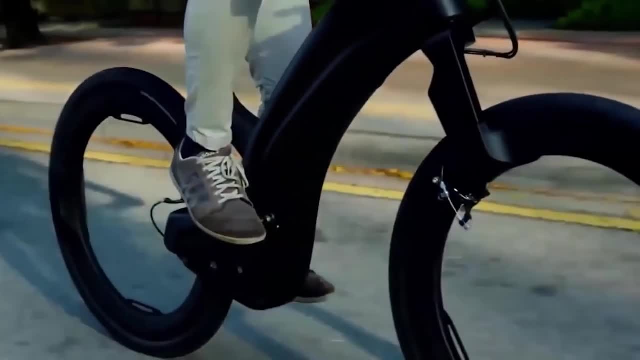 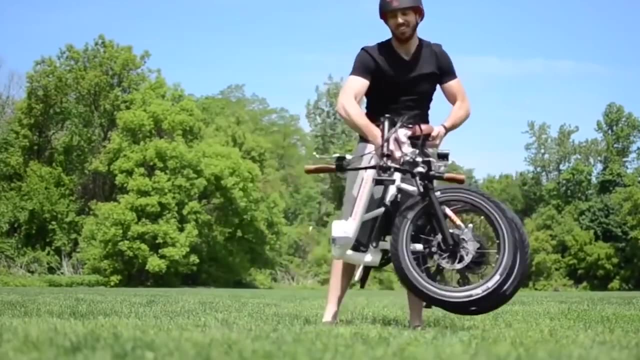 With its pedal-assisted feature, you can cover any type of terrain with ease. E-bikes are fast becoming a highly effective mode of transport with a special capability to solve multiple problems. For context, e-bikes produce zero emissions, improve physical fitness, have long-distance. 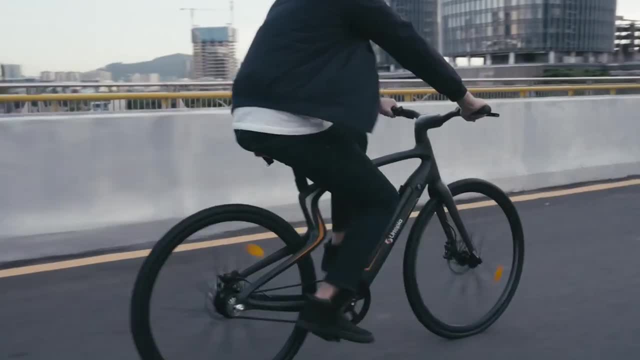 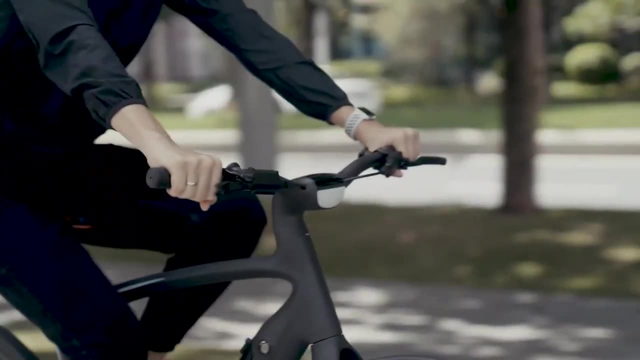 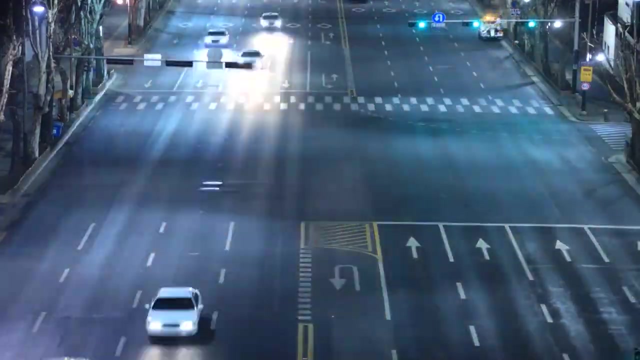 coverage and can reach speeds of up to 20 miles per hour. So whether you want to increase the speed of your e-bikes or increase the speed of your e-bikes, you can only go right with an e-bike. With the success achieved so far, there'll only continue to be more innovations and advancement. 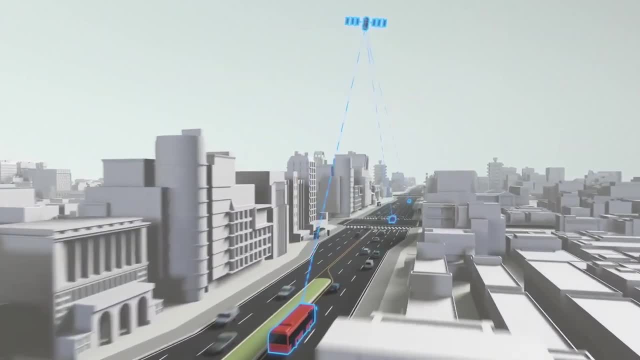 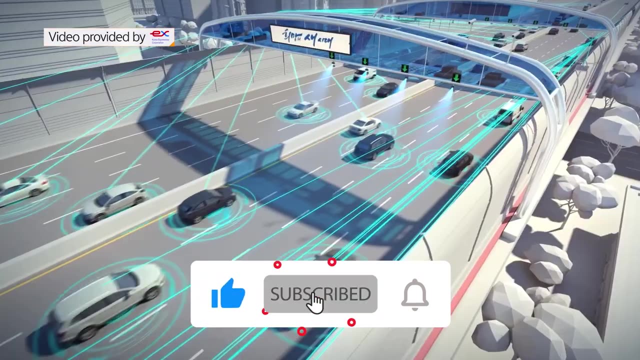 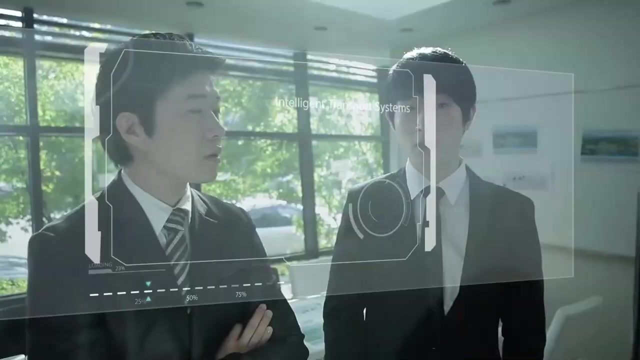 in transportation technologies that'll further make transit better, faster and more eco-friendly. Make sure to give this video a like and hit that subscribe button for more intriguing tech content like this one. Check out this video here To uncover some of the coolest gadgets to make you have a better flight experience.